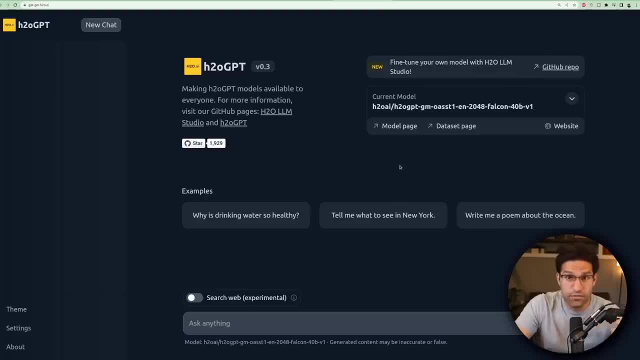 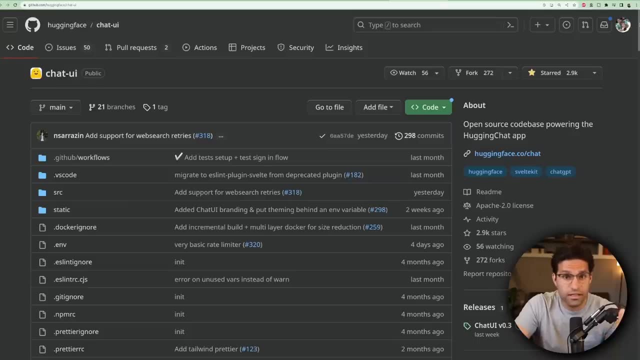 and it provided the answers. The second link is just a different user interface and you can see it looks very similar to other chatbots that you might be used to working with. The back end of this version uses the chat UI interface provided by Hugging Face in the repo. 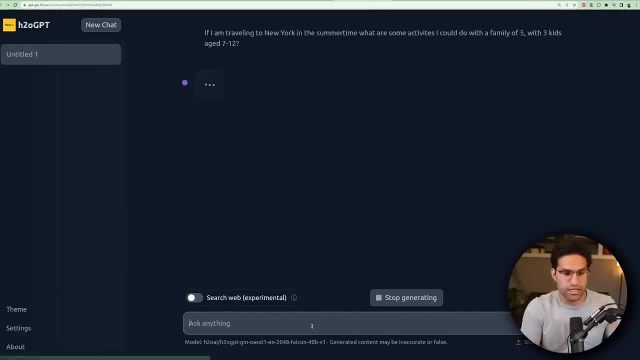 that I'll link in the description. I'm just going to paste the same question into this user interface and you can see that the answer comes across like this. And you can see that I can see the chat UI interface and I can see the chat UI interface and I can see the chat UI interface. 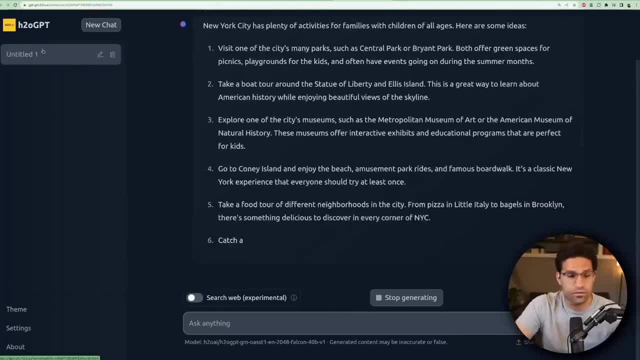 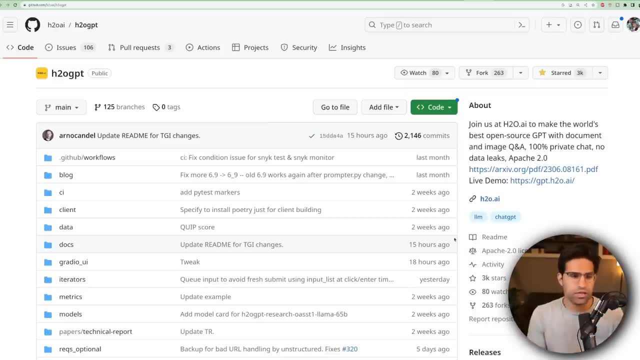 And you also have on the left side a history of all your conversations that you've had. All right, so we're ready to get started loading this code on our machine so we can get it running locally. We're going to start with the H2O GPT GitHub repo. You can see here it says it's 100%. 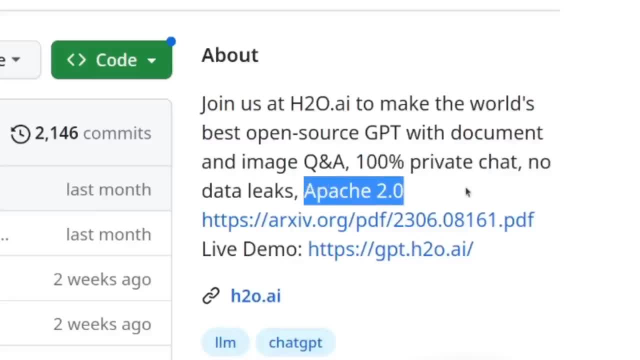 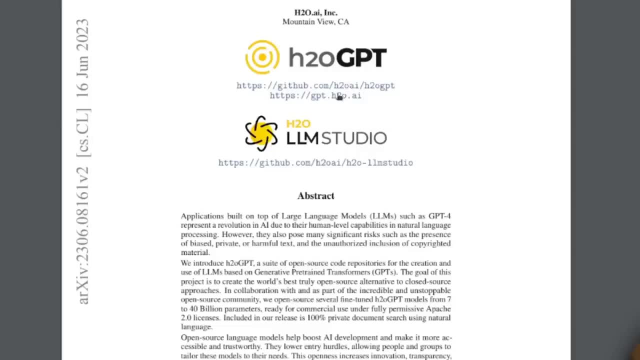 private chat. no data leaks and it's released under Apache 2.0.. There's also a link to the H2O GPT paper that was released. with this code, You can see that it links to H2O GPT. 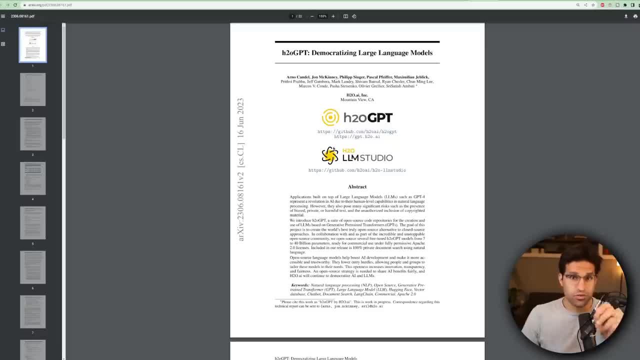 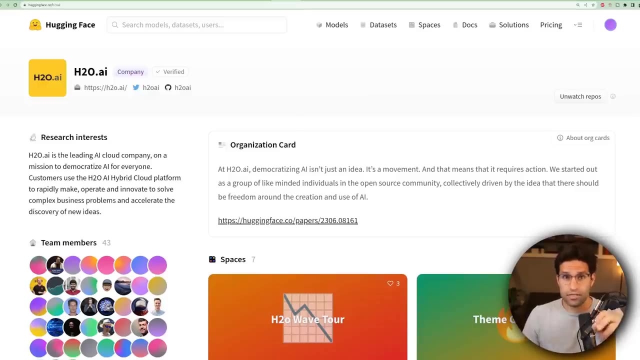 which we're going to install. It also talks about LLM Studio, which is a code base that's used for fine tuning models, and it was used to fine tune the models that we are going to be running today. Now, in addition to the GitHub page, there's also an H2O Hugging Face. 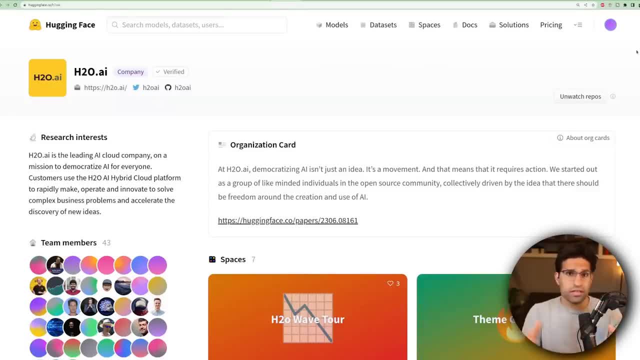 page. Hugging Face website is almost the equivalent to GitHub when it comes to hosting models and model weights. So if we scroll down here on H2O's Hugging Face page, we can see that there are a bunch of different GPT models that are available for us to run. It might. 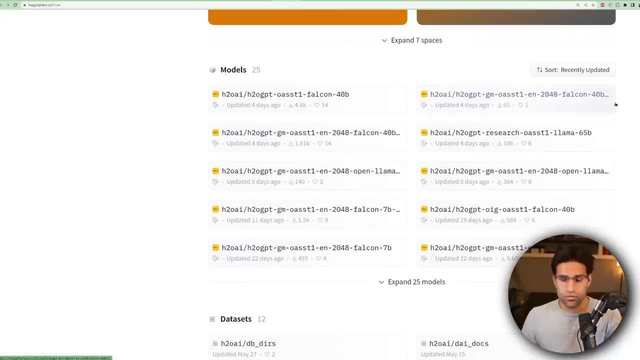 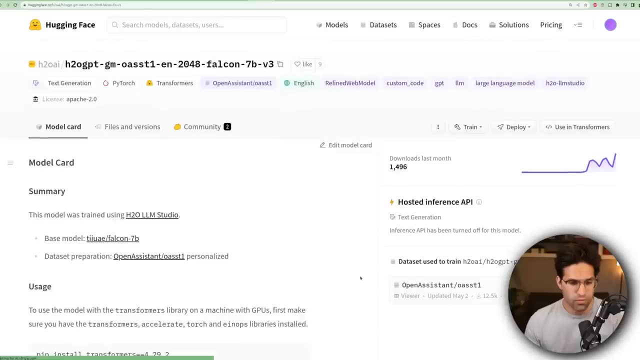 be a little confusing at first for you to decide which one to actually run on your machine, but the name of each model actually gives you a lot of information about what the model is and why you might want to use it. So I've clicked here on this model, which is the one 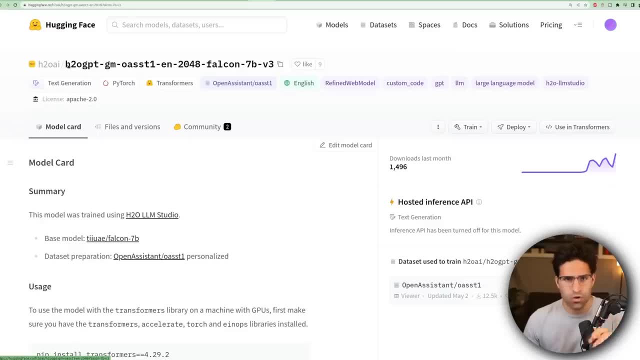 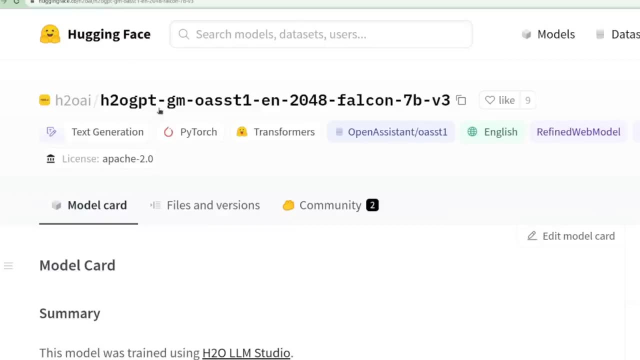 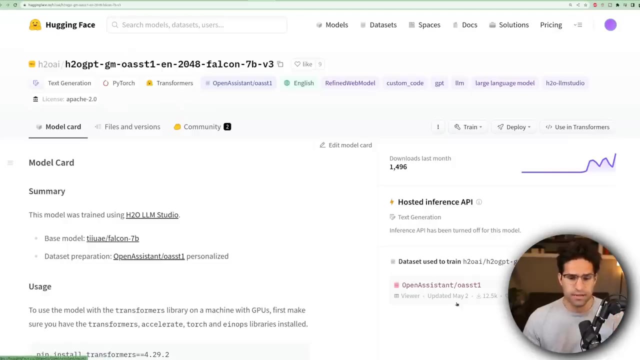 that I'm going to run here on my local machine Just to break down what the naming convention means. this is the H2O GPT model. It's the GM version, which means it was trained by the Kaggle Grandmasters at H2O. It was fine tuned on the Open Assistant dataset. 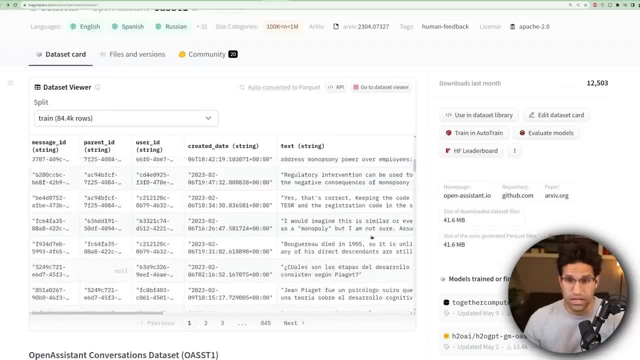 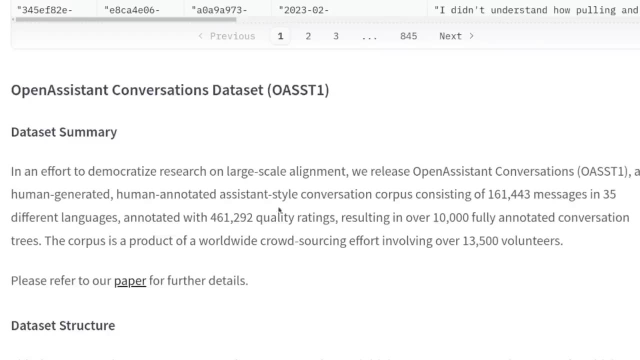 You can also see that datasets here down to the right. Here we can actually see the data it was fine tuned on and read a little bit about the dataset itself. This dataset was designed to be an assistant style conversation. corpus of data. EN means that it was trained. 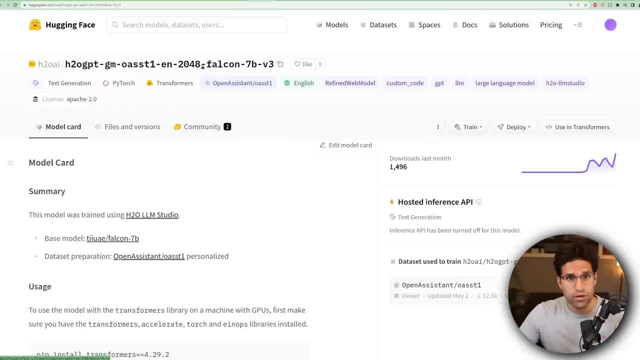 on the English subset of this Open Assistant dataset. 2048 is the number of tokens in the context size of this model. That essentially means how much information can the model take in at one time before giving an answer? By comparison, the GPT-3 model is about 4,000. 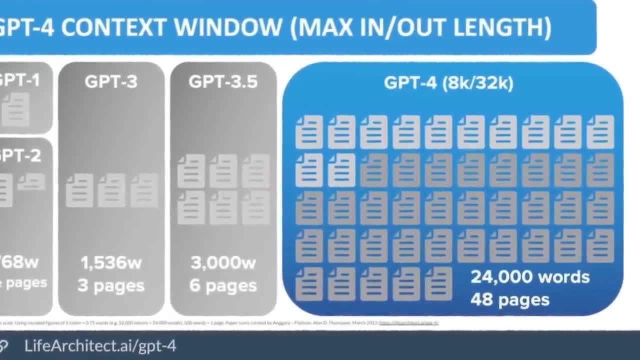 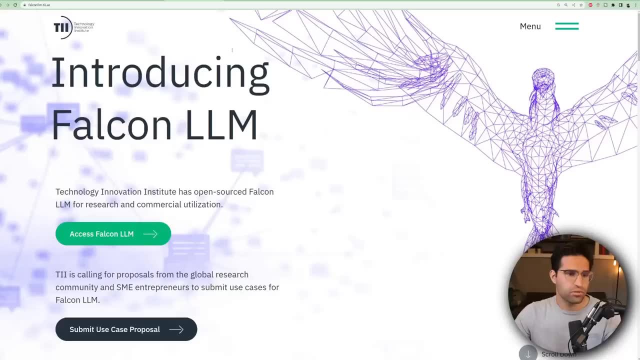 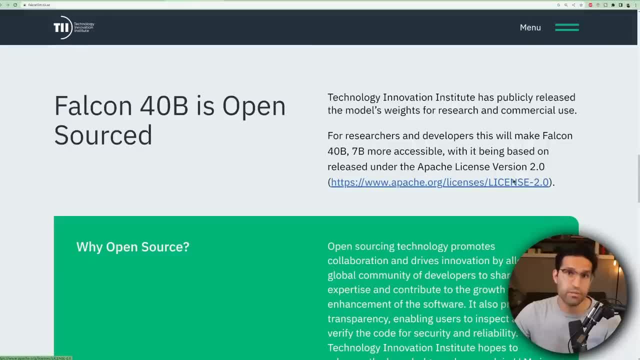 that we'll be running is based off the Falcon 7 billion parameter model. We should probably open source and they're transparent about the data that the model was trained on. By going to the Hugging Face page of this model, you can see that they. 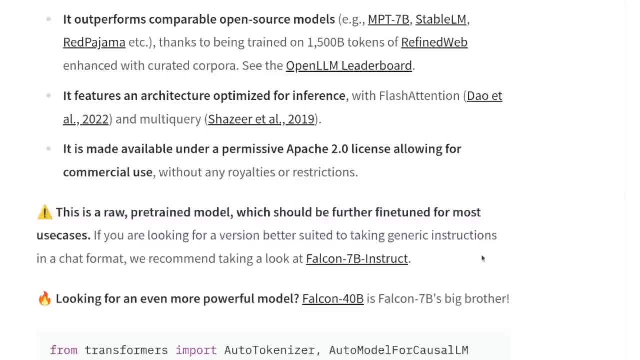 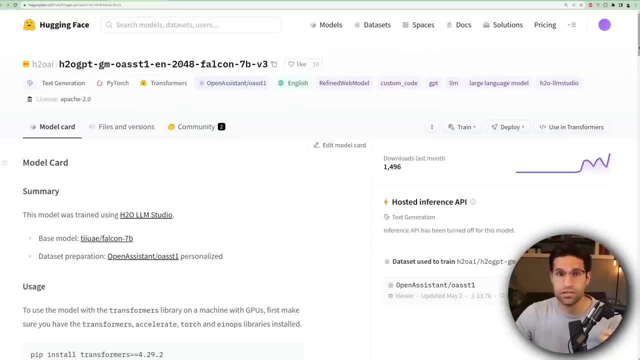 say that this is a raw, pre-trained model which should be further fine-tuned for most use cases, And that, in fact, is why we're using the H2O GPT version of this model, because it was fine-tuned to be a conversation bot. When I showed you the 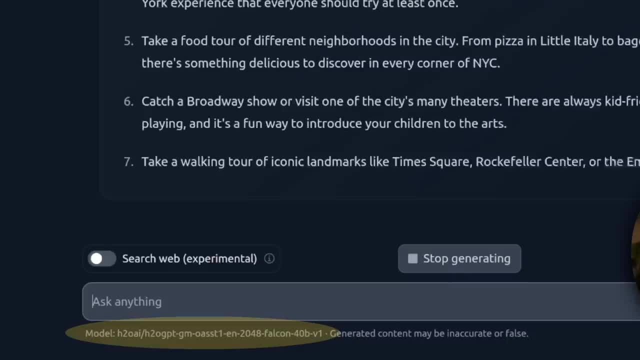 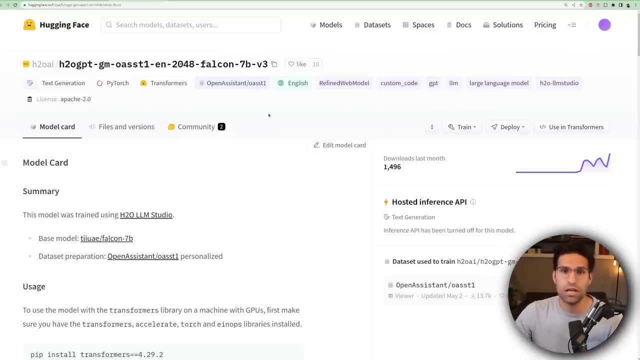 examples. earlier, we were using the 40 billion parameter model and we'll be running the 7 billion parameter model on my local machine because the size of the model requires a larger GPU And my GPU just isn't big enough to fit the 40 billion parameter model. If you don't have a GPU, you could always spin up an 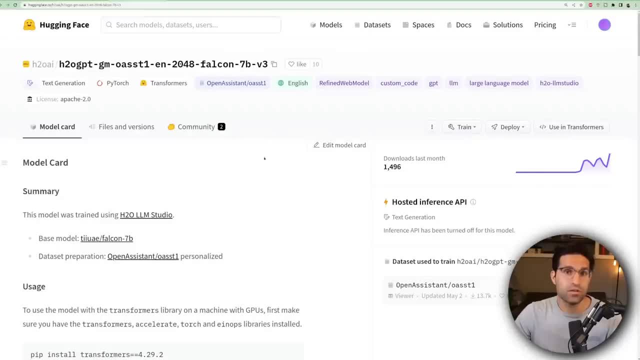 instance, using a cloud provider. if you wanted to- and maybe I'll make a video about that in the future- Just let me know in the comments if that's something that interests you. Another thing that I've been doing is I've been working on a lot of my 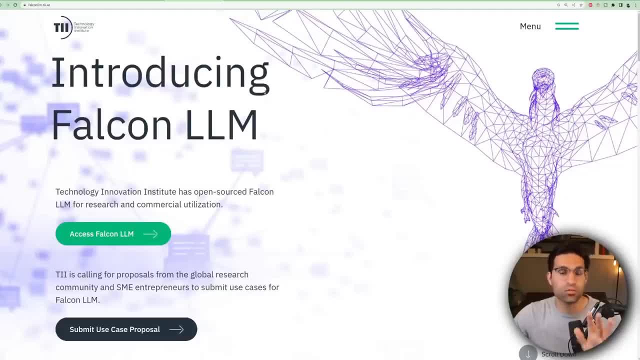 testing on these H2O GPT models, and I've been doing a lot, of, a lot of testing on these H2O GPT models, And one other thing I'd say about these foundational models is that things are moving really fast and new models are coming out. it. 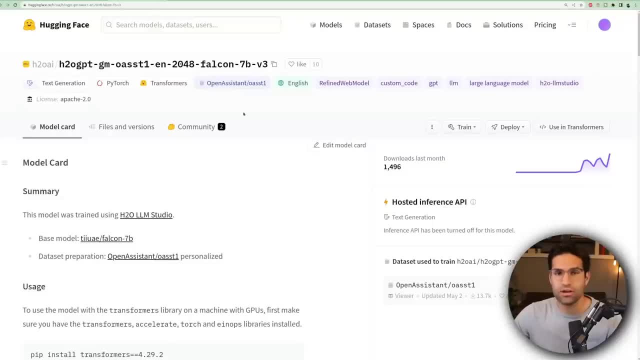 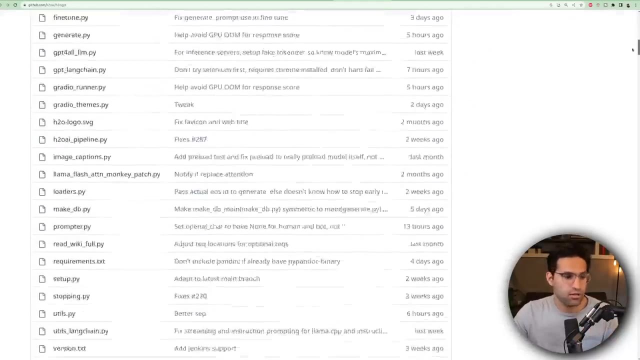 seems like almost every month. The nice thing about using these H2O models is that the team that works on it is dedicated to testing out all these new open-source models and fine-tuning them for specific tasks. Going back over to the H2O GPT GitHub repo, if we scroll down we can see the README document has. 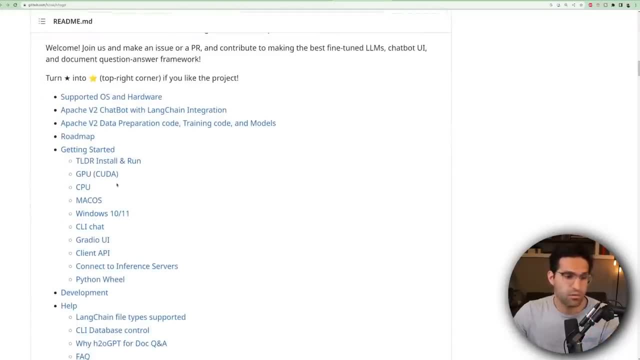 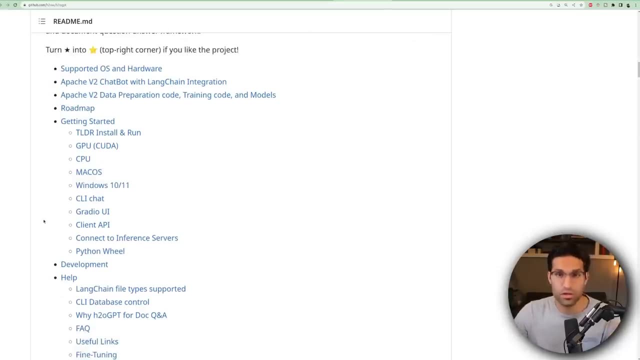 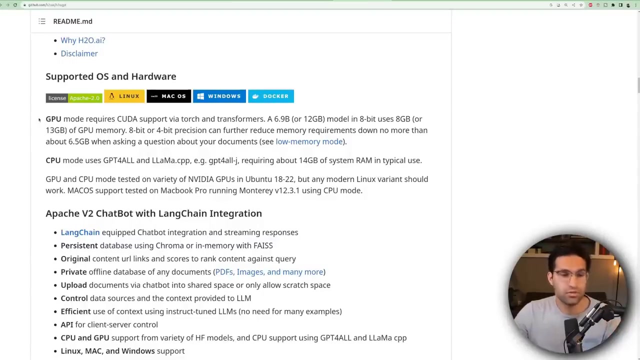 instructions for how to install this on a bunch of different objects: operating systems. you can install it on Mac or Windows, and we're going to be installing it on my machine that's running Ubuntu. I already mentioned this before, but if you want to run these bigger Falcon models, you're going to need a GPU, and specifically one that can run CUDA. 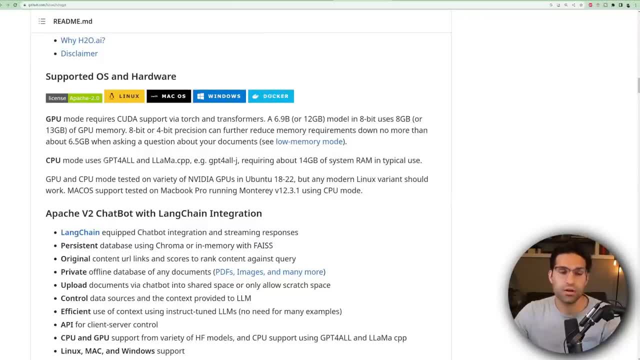 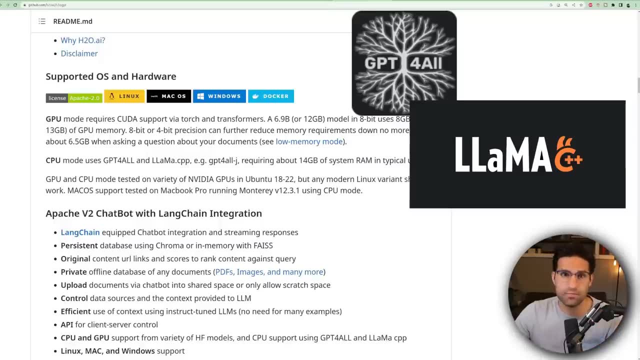 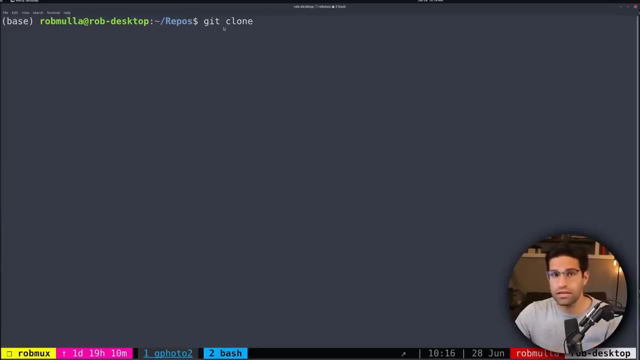 If you just want to give it a try, there are some models that you can run using CPU mode, like GPT for All and Llama CPP, and you would just have to follow the CPU instructions if you wanted to run it that way. So, jumping over here to my terminal, the first thing we're going to want to do is git. 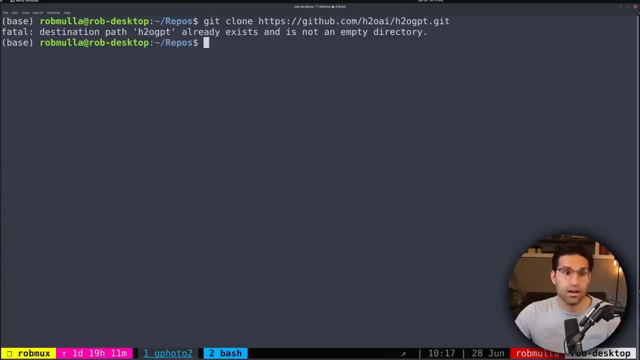 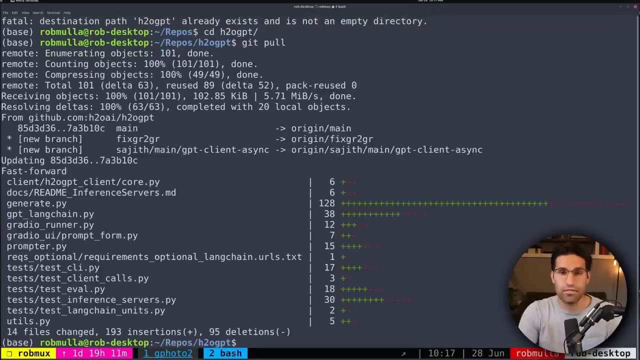 clone the h2ogpt repo. Now, for me I already have that cloned, so there's a directory called h2ogpt, but for you it would just download the code into whatever directory you are in. Now we can cd into that directory and I'm actually going to run a git pull just to make sure I have the most recent. 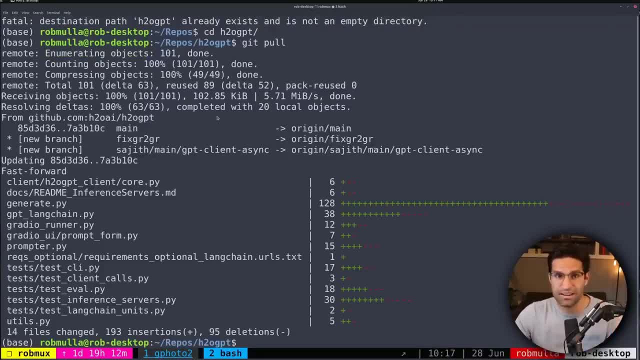 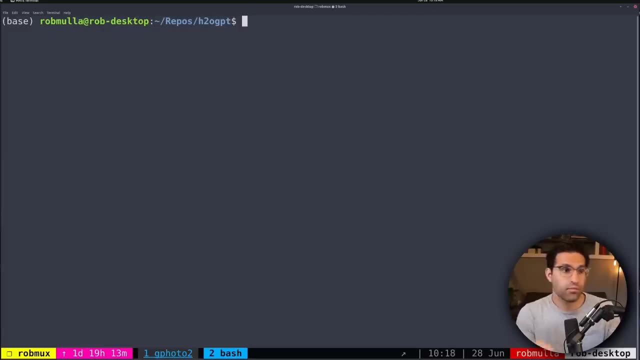 version of this repo. This codebase is in active development, so a lot is changing each day. If you run a git pull, you'll pull the latest version of the codebase. The next thing you'll need to do is install the necessary packages to make sure that h2ogpt can run. Whenever I'm 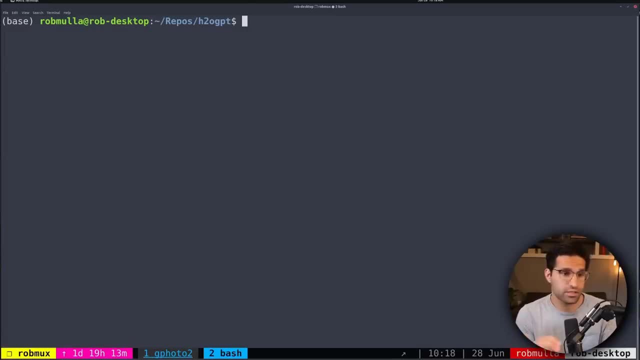 working on a new Python project that involves installing specific packages. I like to create a brand new environment where I install those. There are different package managers out there, but I like to use Conda. You can install miniconda or anaconda on your computer if you don't have that already. 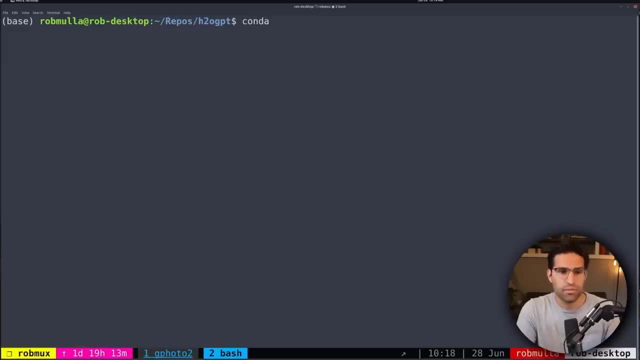 and that will allow you to create a new environment. I do that by running conda create, then I provide the name, which is going to be h2o, gpt, and then I'll tell it the python version that I want, which will be 3.10.. Now it's telling me the conda environment already exists, so I'm just going. 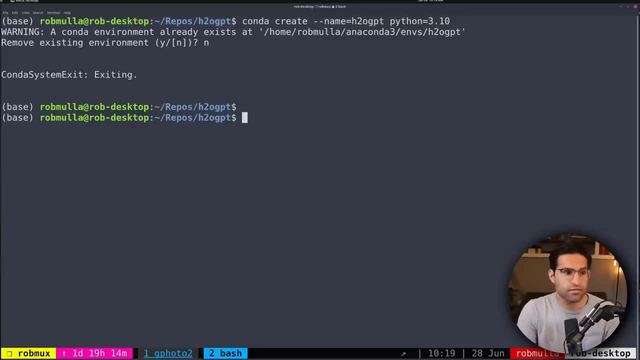 to hit n here, but for you that would create a new anaconda environment and then we can activate that environment by running conda conda activate h2o gpt To install all the necessary packages. we are going to use pip by running pip install and then dash r the requirements dot txt file To be clear what. 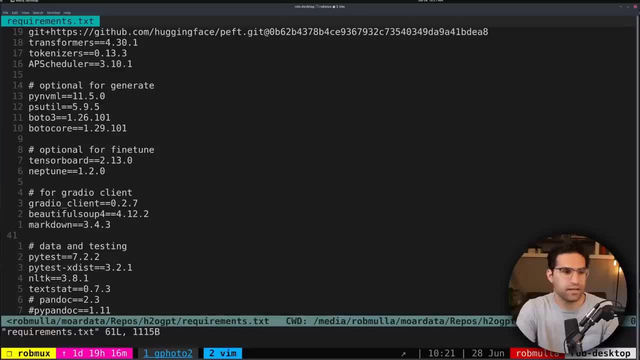 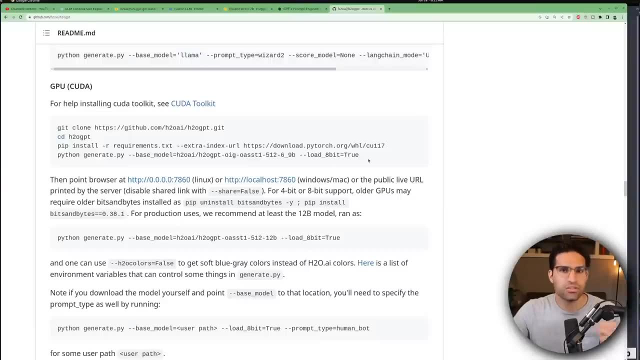 that's installing. we can look in this requirements txt file. Here we can see all the dependencies that are required in order to run h2o gpt And, following the instructions from the readme document, you can see that they recommend also installing the h2o gpt file If you want to. 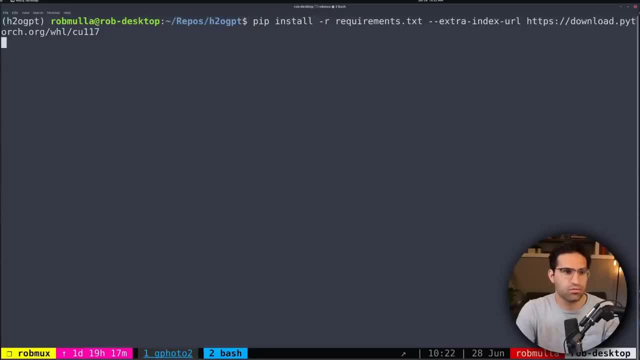 run h2o gpt in this extra index. so we're just going to paste this whole line and run it in this conda environment. Now that that's done, all the required packages have been installed. Another thing you want to check is to make sure that you have CUDA installed. I can check that by running. 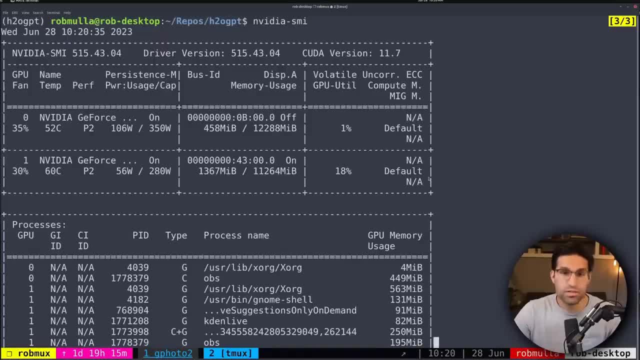 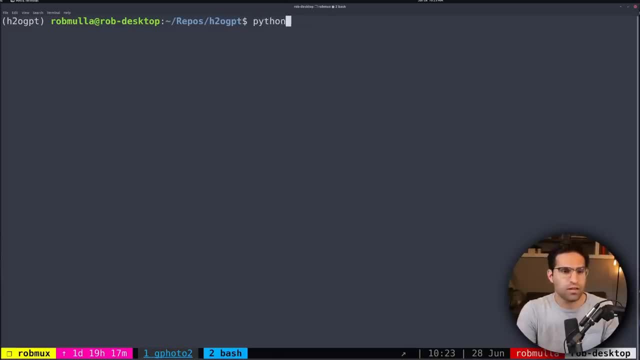 nvidia smi and it'll show all of the GPUs I have on my machine and that CUDA version is installed. Now we can test running this model by running python generate, and there are a few arguments we're going to need to provide so that we can run this model. So I'm going to run this model. 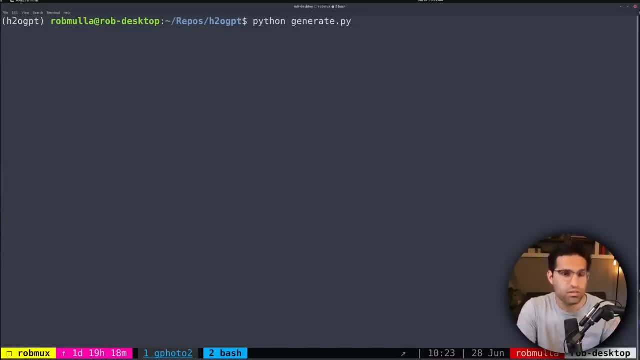 h2o. gpt knows which model and how we want it to run, So we're going to provide it a base model, and that's this version 3 of the falcon 7b model, So I'll paste that in here. We're also going to 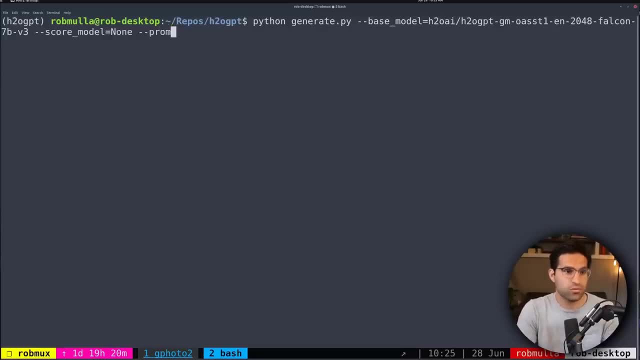 say, score model equals none. We're also going to tell it the prompt type, which is going to be human bot. And for our first test, we're just going to run the command line interface version Now, before I hit enter on this. if this is your first time running this command, it's going to actually 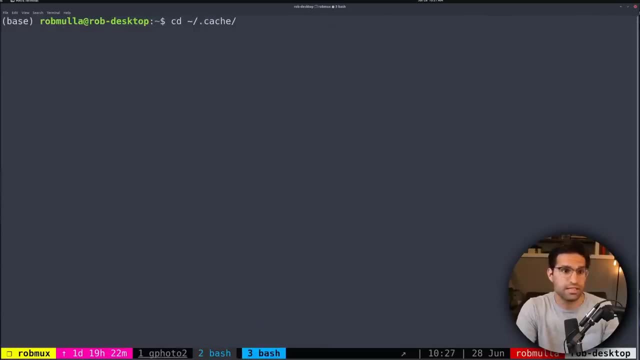 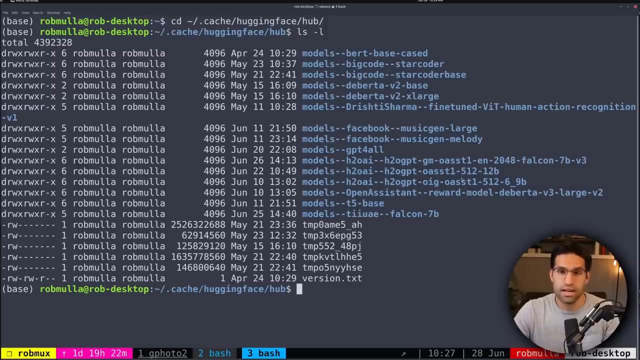 take some time. Just to show you, if I cd into my cache directory under hugging face hub, in this directory we can see that all the models that I've tested out have been downloaded and I can enter into the directory with the model that we're going to be running now. 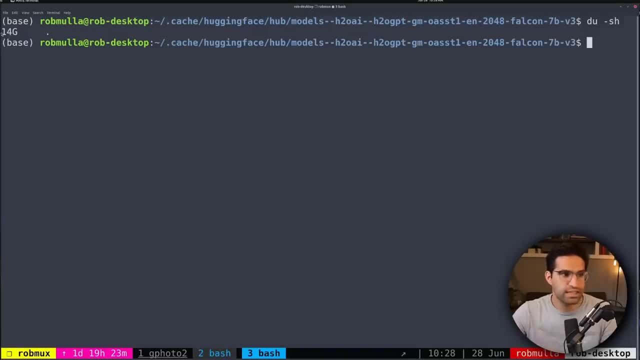 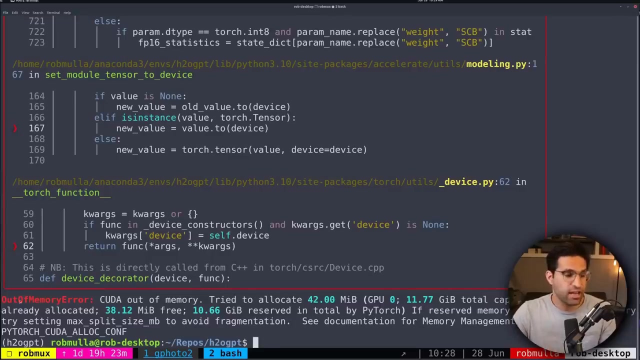 And by running du-sh, we can see that this model has a total size of about 14 gigabytes. So back to this command that we're running. I'm just going to hit enter on it and you can see that it's loading the model weights into my gpu And we actually get an error here and this is an. 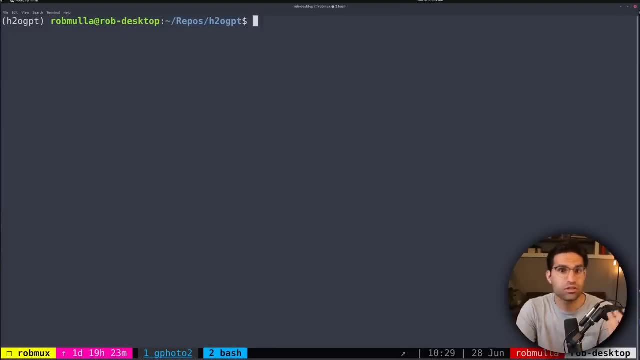 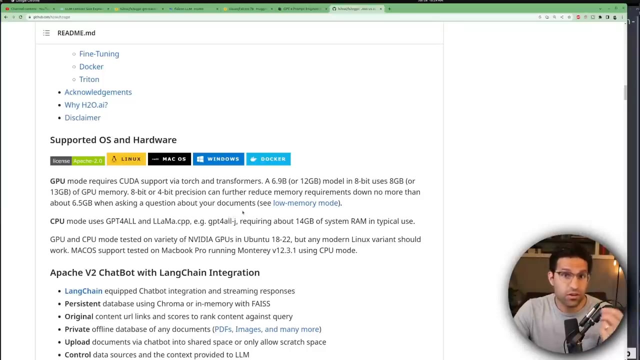 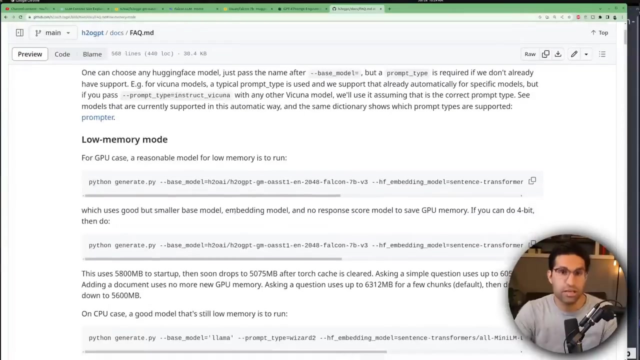 out of memory error. That's because this model is too large to load on its own into my gpu on this computer. But luckily there are some tricks we can use to get large models into gpu of certain size memory And there's a whole section in the documentation about how to do this. But essentially 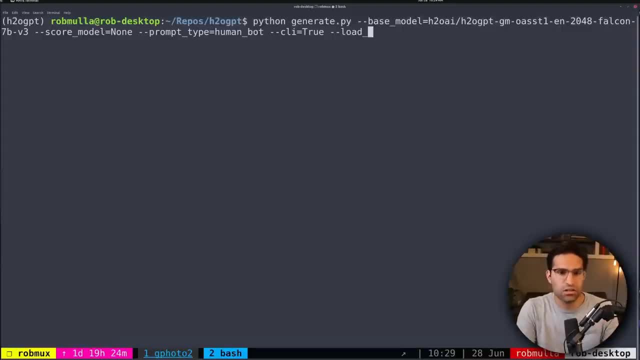 what we're going to do is add to this generate call a load 8-bit version of the model, And this will load the model into our gpu memory in a more efficient way. If I create a new tab here, I can show you that it's now loaded into my first gpu's memory and it 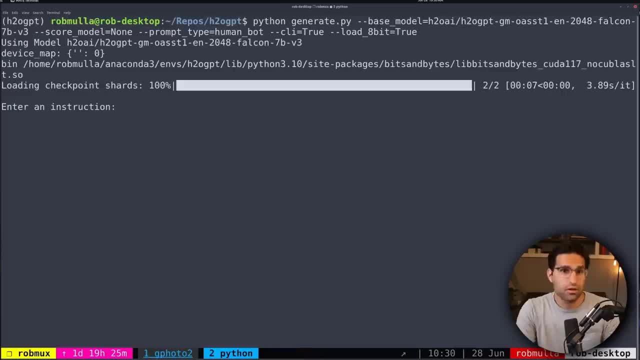 has 9.2 gigs of memory being used, There may be an impact to the quality of the model responses when you run this quantization- 8-bit or 4-bit- on your models. Since this is a conversation bot, we can ask a question like: what is the purpose of having large gpu? 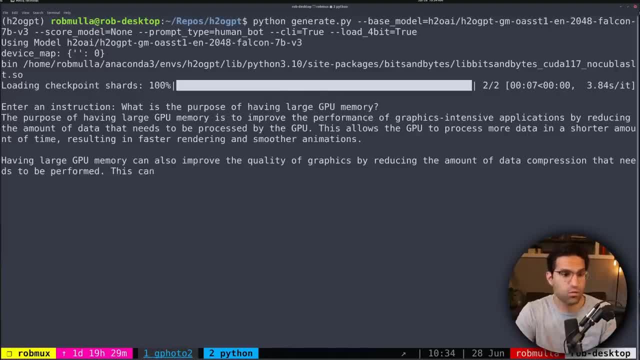 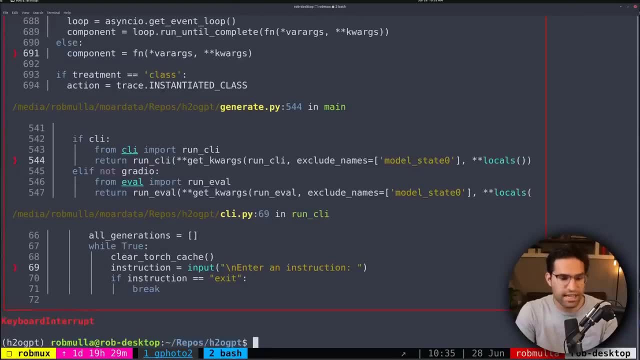 memory And you can see it's providing us a nice answer for why you would have large gpu memory. So it did a pretty good job at answering that question. Now I'm going to hit ctrl-c to exit out of this And we're going to run the graphical interface version of this model. 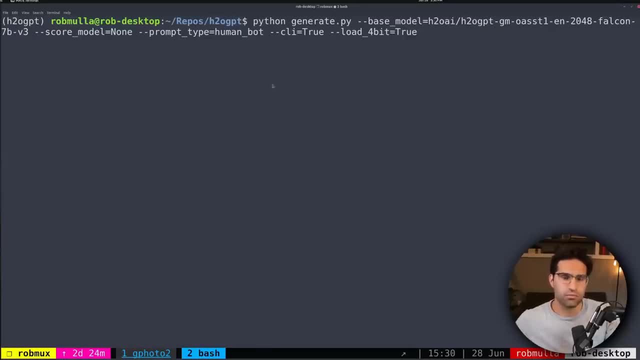 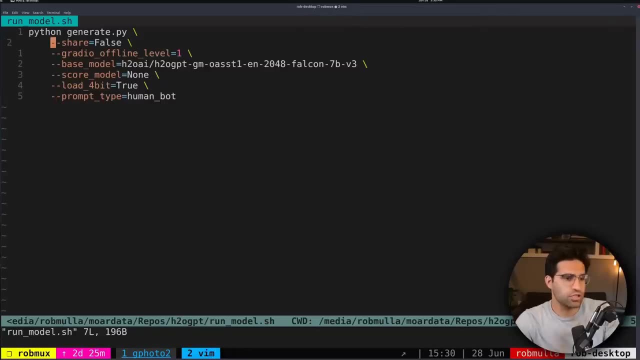 Now one thing I like to do. since this line of code has gotten pretty long and there are a lot of commands that we're running, I like to create a script that has all these commands in it. I've turned sharing off and turned the offline level to one. This will ensure that the 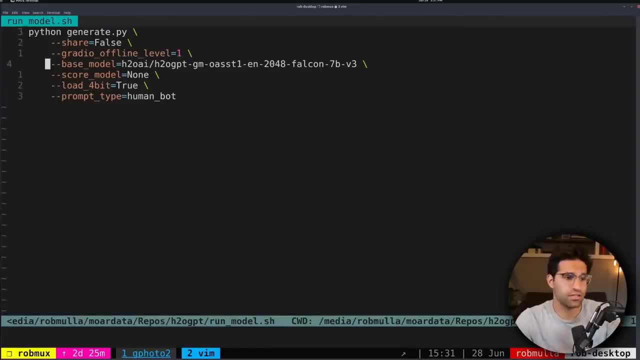 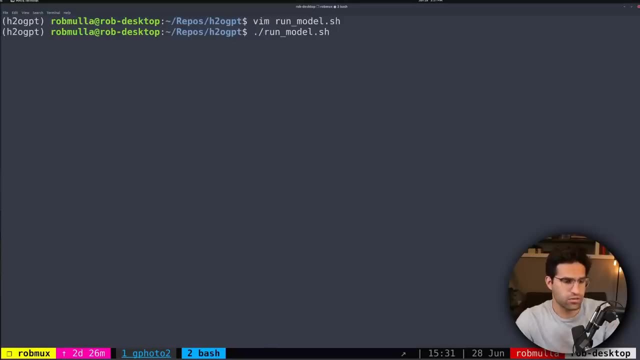 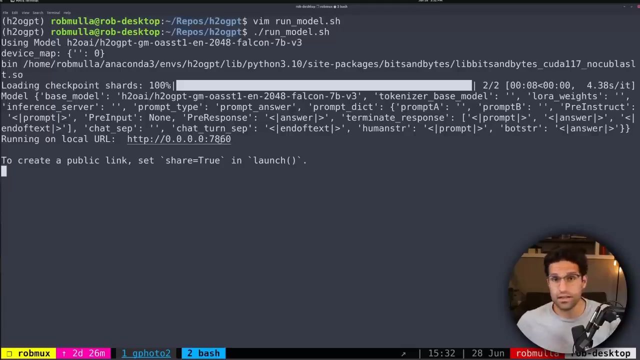 model is running offline And you can see that the model and the other settings we have are the same. I've just removed the argument that disabled the UI. So if I go back here and run this script and we could see that it's running on our local machine now on port 7860.. So if I click on this, 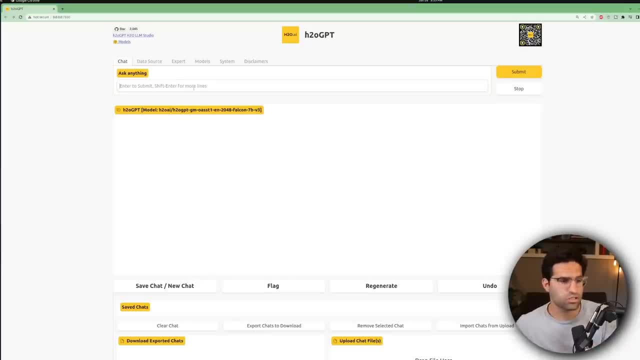 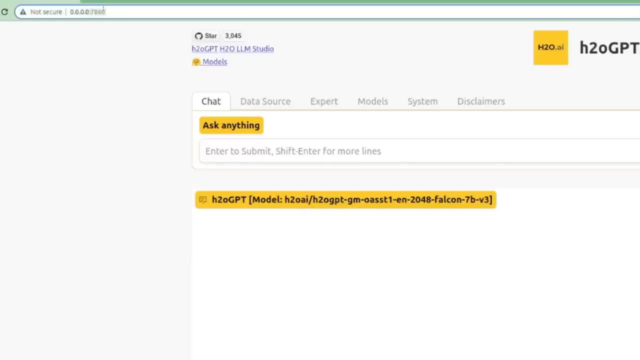 or open this url in a browser. I'm taken to this page, which looks very similar to the h2ogpt site if you went to it online, Except for it's running completely on my local machine Now we could see that. it also tells us which model that we're running, which is the 7 billion. 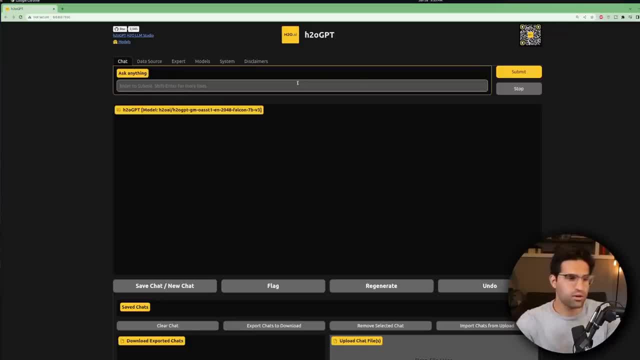 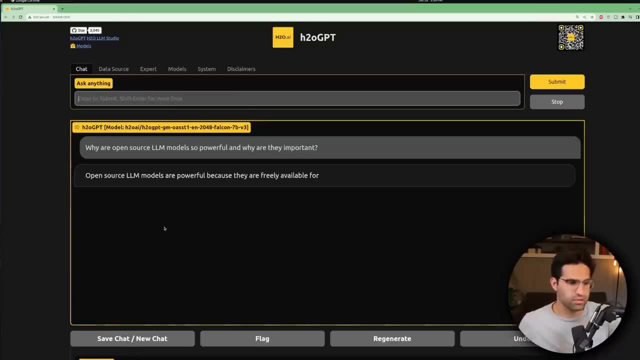 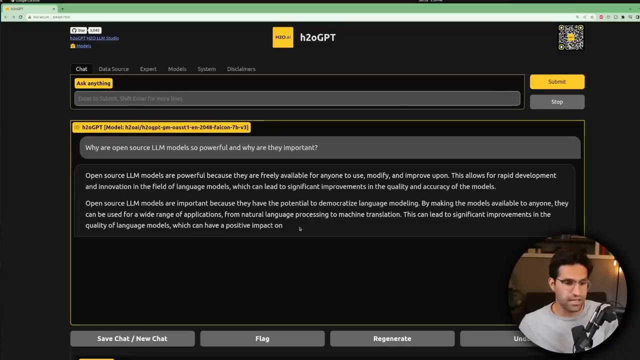 parameter falcon model. I can go ahead and enable dark mode and let's ask it a question. I'm going to ask it why open source llm models are powerful and why are they important. Open source models are powerful because they are freely available to anyone to use, Allows for rapid development and 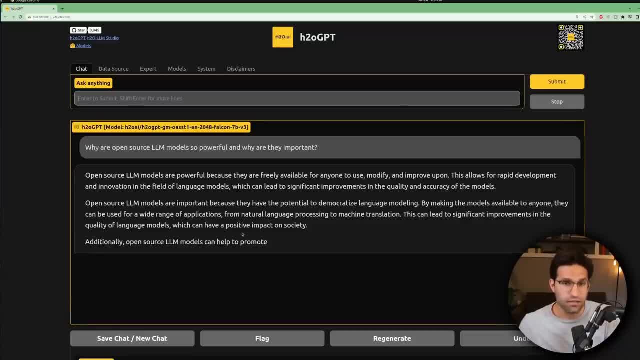 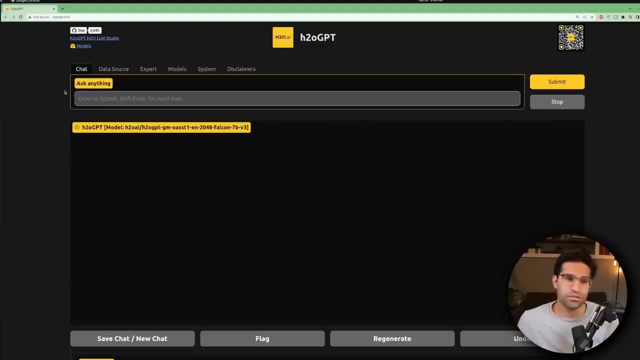 it looks like it's running fine. It's a little bit slower than the online version because my gpu isn't necessarily the fastest, And the answer is done. Like I said before, this user interface is undergoing some rapid development so it may change, But one of the nice features I like about it is it's integrated. 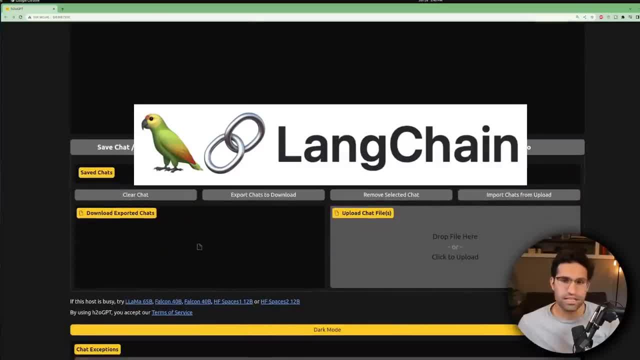 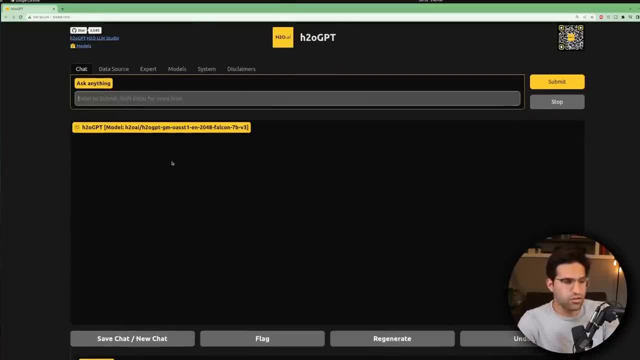 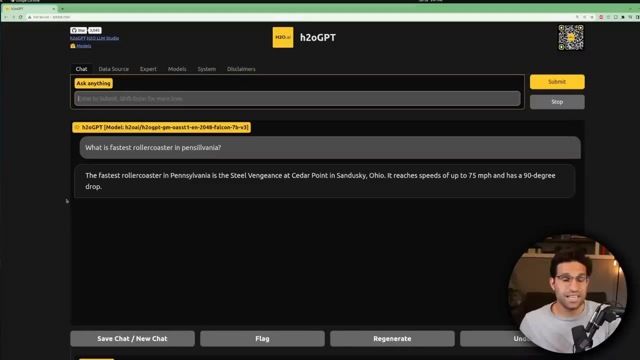 lang chain which allows you to actually import data sets that you might want the model to use in order to provide a better answer. A nice example that I tried before was asking the model: what is the fastest roller coaster in Pennsylvania? You can see it gets confused here. 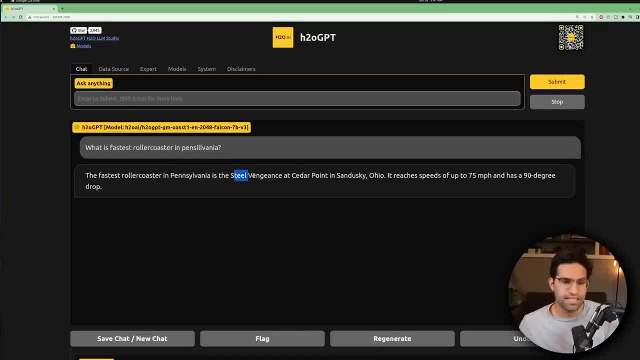 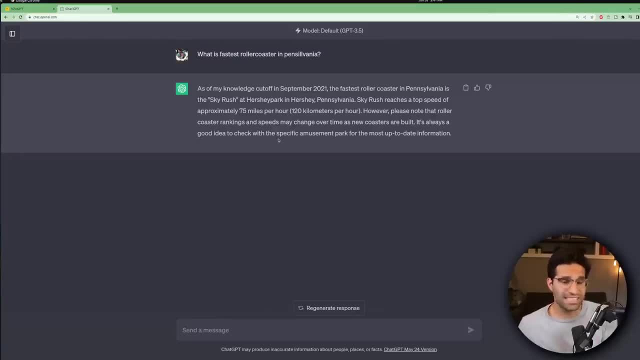 and it says the fastest roller coaster in Pennsylvania is the steel vengeance, but then it says that it's in Ohio. So we know this isn't correct And, to be fair, if I ask the same question of chatgpt 3.5, it gives the wrong answer too. It says it's skyrush which is in Pennsylvania. 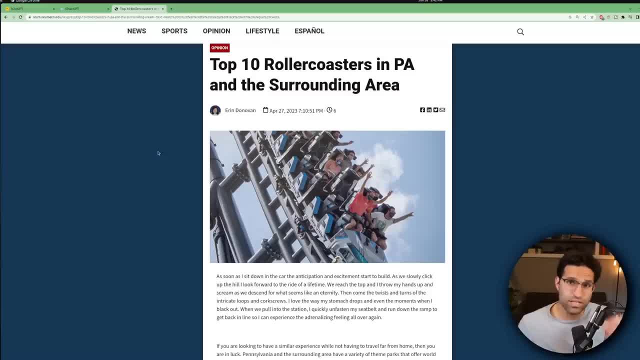 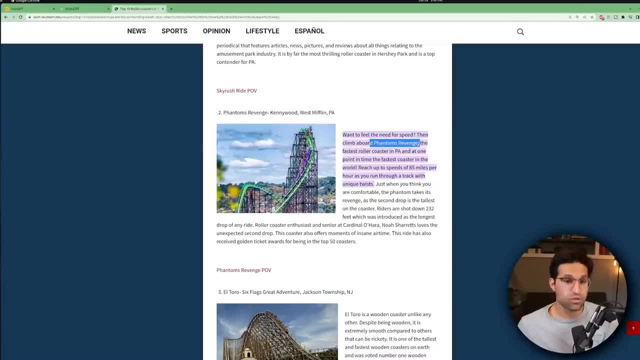 but it's not the fastest roller coaster. So I found this recent article that does mention the fastest roller coaster in Pennsylvania is this roller coaster called phantom's revenge. I'm going to take this article and save it as a PDF to my computer. Then I'm 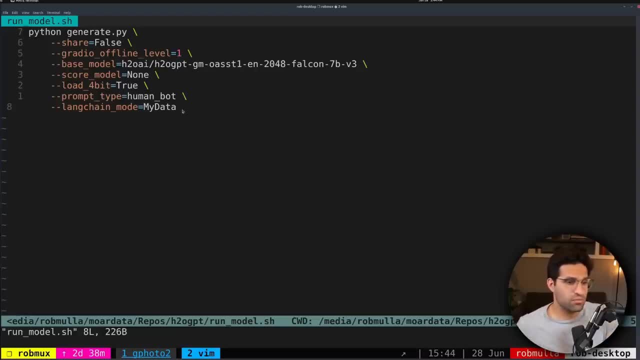 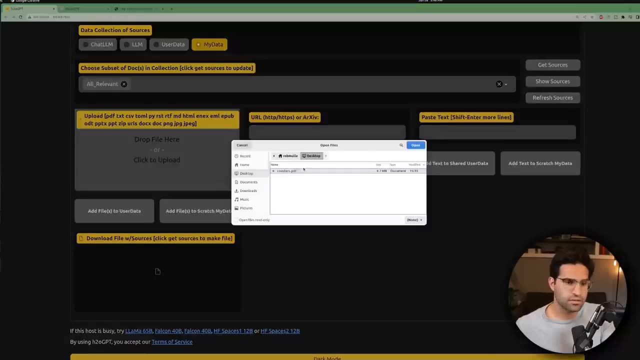 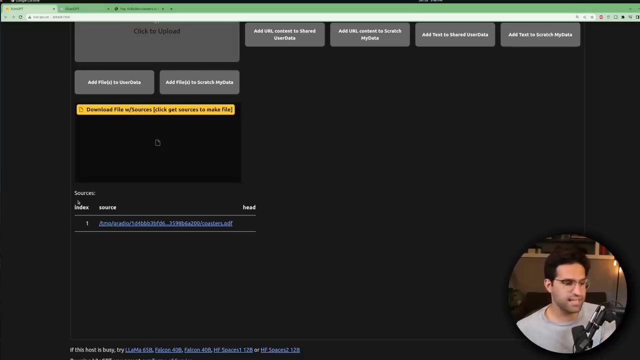 going to reset H2O GPT with this lane chain mode set to my data. Now that it's reset, I can go to this data source tab and I can click here to upload a file and click add files to user data. What this is doing on the back end is creating a vectorized database entry with this coaster's PDF. 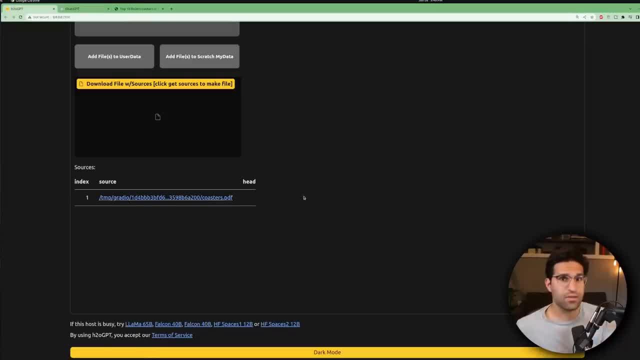 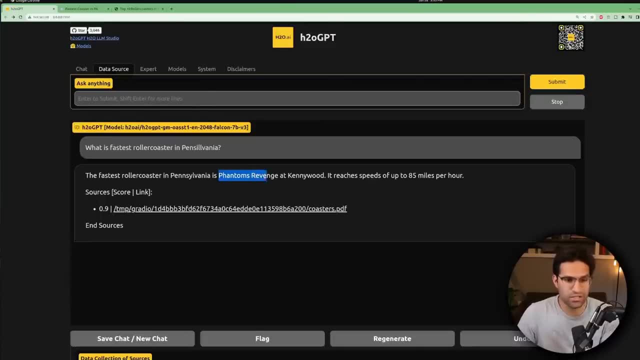 So now this data source can be used by the LLM to help answer my question. Now, if I ask the same question again, we can see that the answer is correct. Now it gives the correct roller coaster. It also links us to the file where it found the result. This still is an experimental feature. 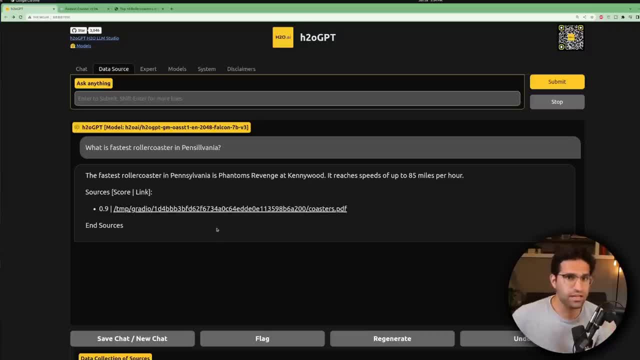 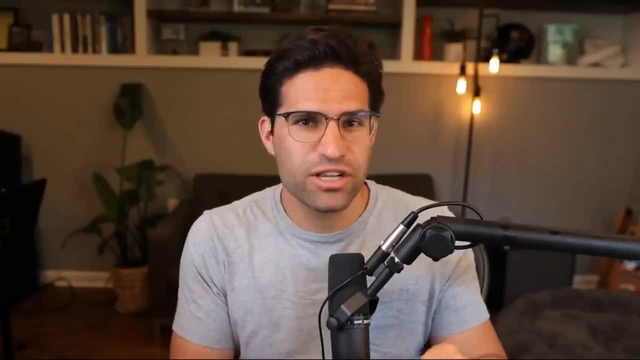 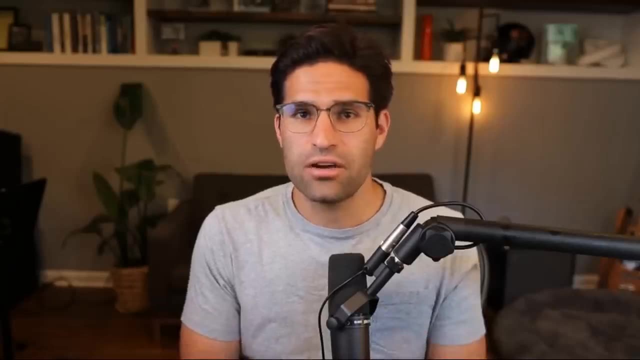 and its ability to search really large sets of data is limited, but at least for this example, you can see how it might work for a future application. I just want to address the question that you might be thinking, which is: why would anyone even want their own open source large language model? I don't necessarily think. 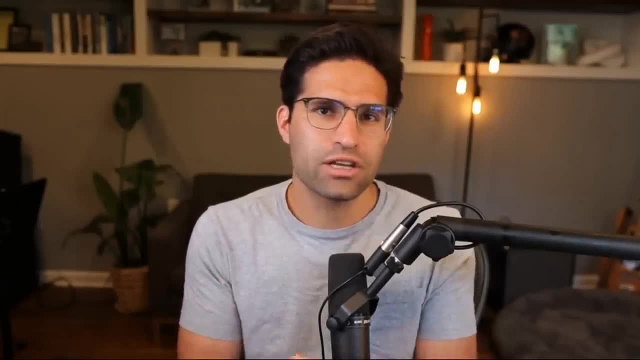 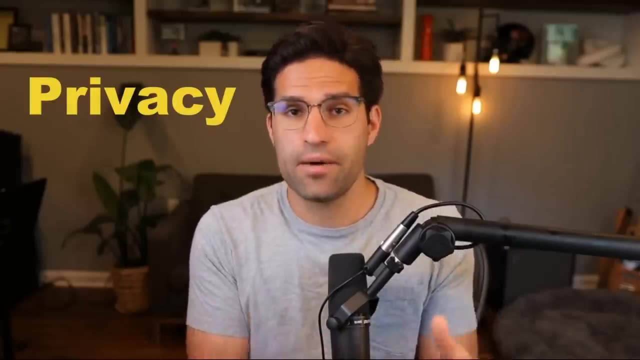 there's one answer to that question, but there are a few things that you should keep in mind. The first one is privacy. Whether you like it or not, anytime you type in any question to a chatbot, that data is being sent somewhere and potentially stored and used. There have been reports about 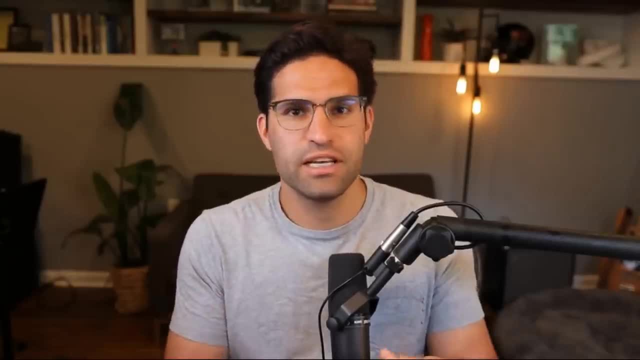 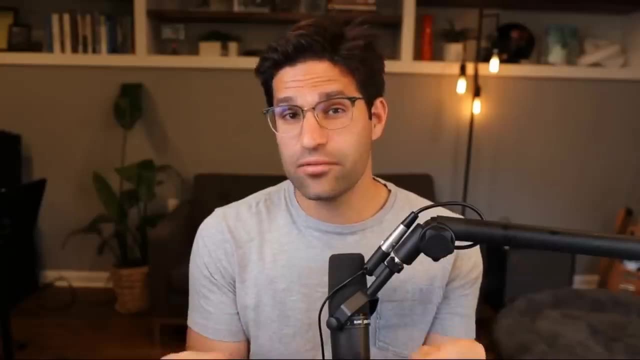 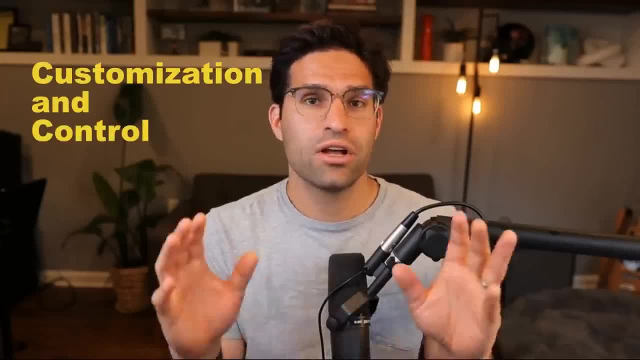 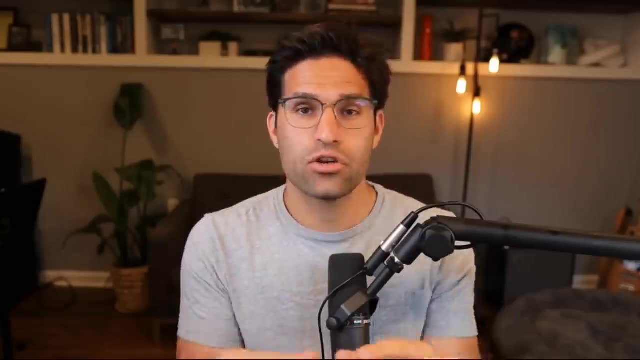 and that's the ability to customize and control your model. Right now, you have a bunch of options for models that are good at answering almost any question. The great part about open source models is that you're able to take those model weights and fine tune. 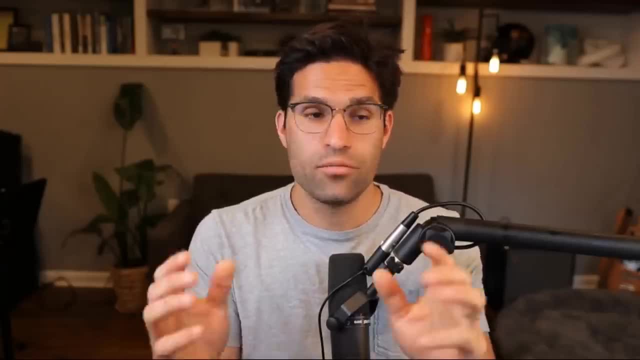 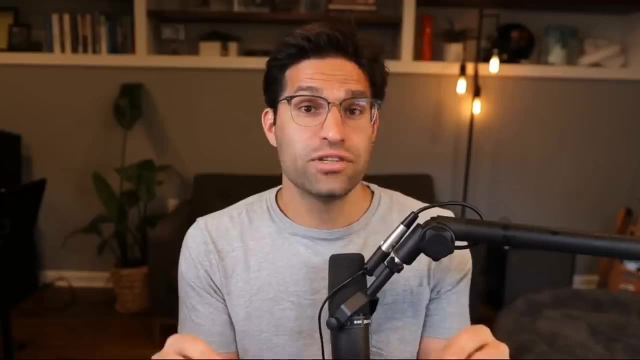 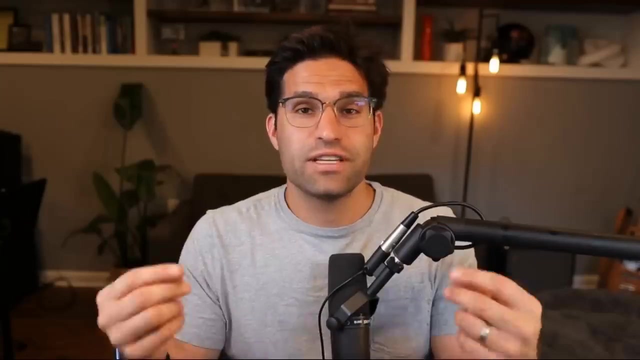 them on any particular tasks that you're interested in. You may have already seen this, where models have been trained specifically for health care or for financial advice. using an open source model, and specifically one that allows commercial use, opens the door for developing a wide range of these custom models, and really i think this is 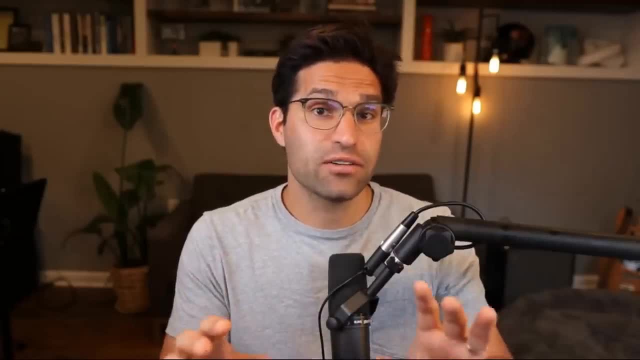 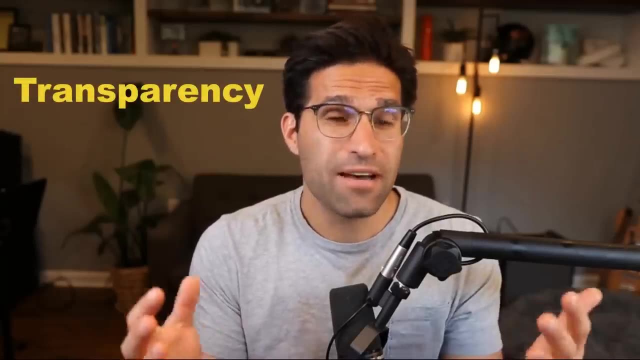 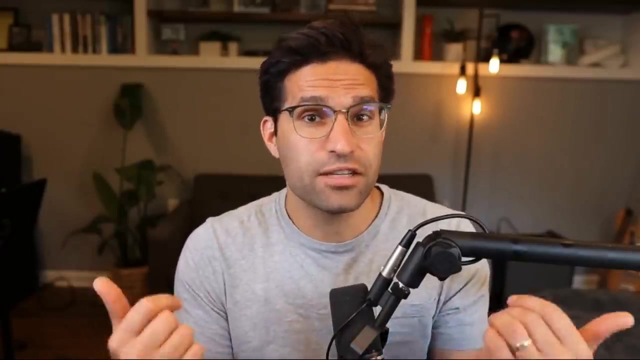 where we're going to see the most advancements in large language models in the years to come. and the third reason is transparency. large language models, like most models, may have some biases. they also can be overconfident and just give wrong information. open source models still have these problems, but at least you know exactly the data that the models were trained on. 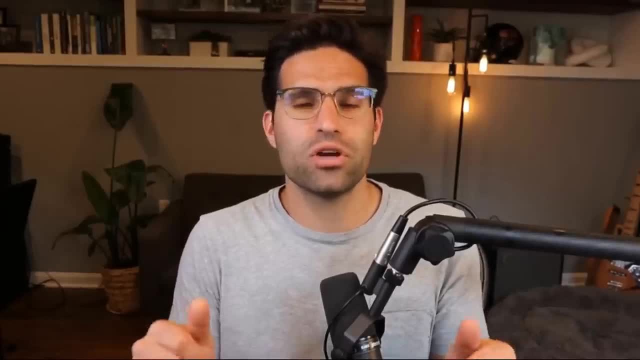 and how the training was done. thanks for watching this video. let me know what you thought of it and i'll be back again soon with another one.